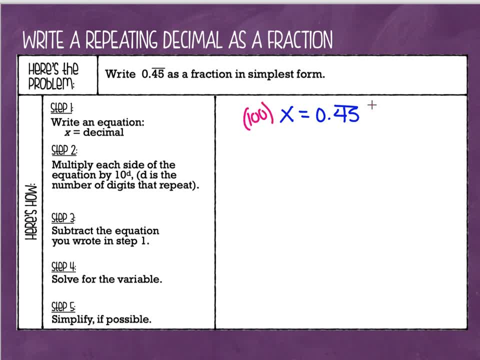 side of my equation by 100. So I'm going to multiply the left side by 100 and I'm going to multiply the right side by 100.. Now, when I do that, I'm going to get 100x on the left side. and if I were to multiply 0.45, repeating by 100, that means I'm going to be moving this decimal. 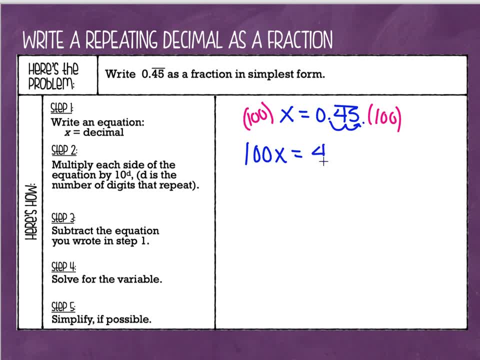 point over two places to the right. So it's going to become 45.45 again, right, because that's repeating. All right, the next step is I am going to subtract the original equation that we wrote in step one. So this equation right here, x equals 0.45, repeating. I'm going to subtract it, I'm going. 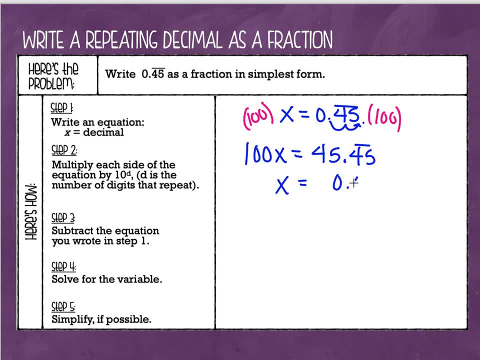 to write it right underneath. I'm going to line up my decimals and I'm going to subtract this equation. If I do 100x minus x, that gives me 99x and I'm going to subtract this equation. And if I do 45.45- repeating minus 0.45, repeating, these two repeating 45s are going to cancel. and 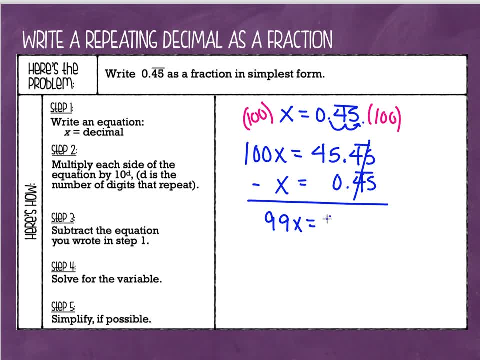 that's what I want it to happen, right? I wanted them to cancel out, and I'm just left with 45.. From this point, we've got a one-step equation left, So let's divide each side by 99.. Now, I'm not really going to divide it, right. I'm going to leave it as a fraction: 45 over 99.. 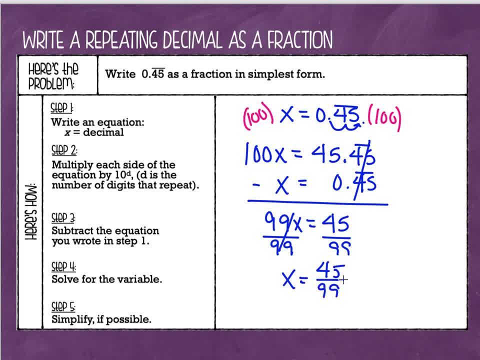 But what I am going to do is I'm going to simplify it. So I'm going to ask myself: what can I divide both 45 and 99 by, Which would be 9.. So if I divide the numerator by 9, 45 divided by 9 is 5.. 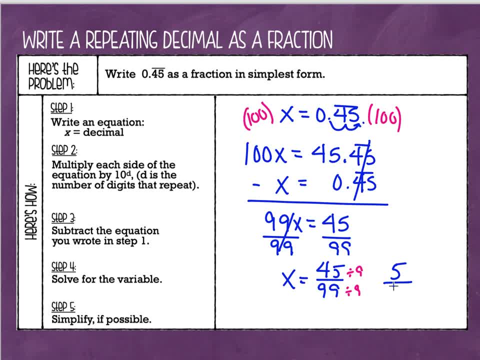 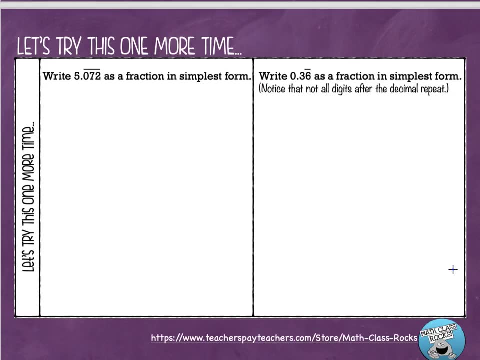 And then if I divide the denominator by 9, 99 divided by 9 is 11.. So 0.45, repeating as a fraction in simplest form, is going to be 5.45.. over 11.. All right, let's do another example. We're going to follow those same steps. 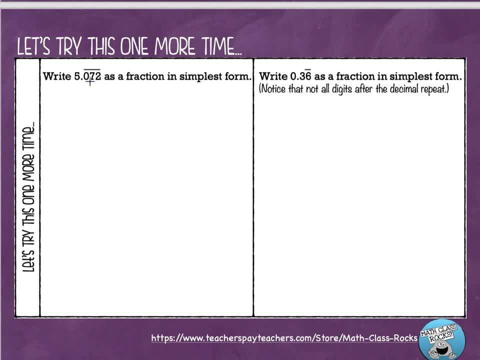 Okay, the first thing I'm going to do is I am going to rewrite this repeating decimal as an equation, right? And I'm going to write x- equals. and then I'm going to write the decimal, Now this five, right here. I'm going to save it until the end, because all that's going to do. 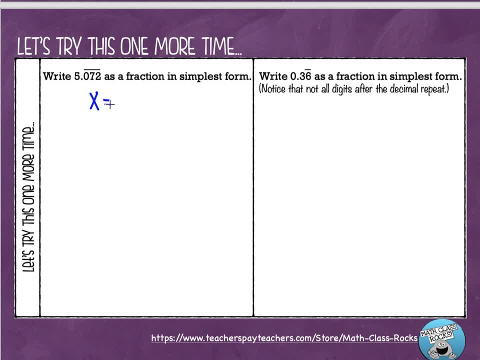 is, give me bigger numbers to deal with, and I don't really want to do that right now, So I'm going to save that five till the end. I'll actually circle it, so we don't forget about it. I'm going to start out by writing just my decimal, and it's 0.072. repeating So x equals 0.072. 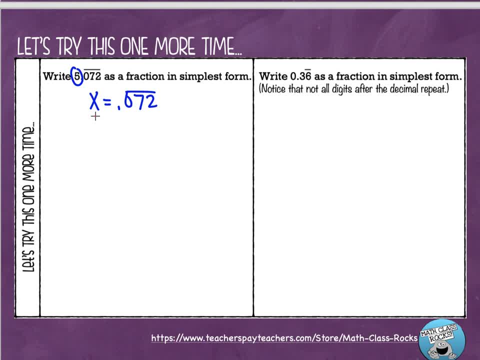 repeating. Now that next step is I have to multiply each side by 10 to the d power right, And that the d power is the number of digits that are repeating. Well, I have three numbers repeating, which means that I would multiply each side by 10.. 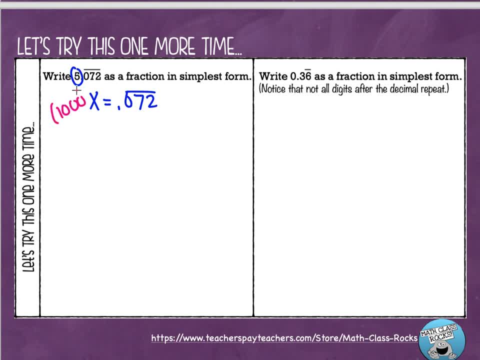 10 to the third power, or 1,000.. All right, 1,000 times x is just 1,000x. And then if I multiply this number by 1,000, I'm going to move my decimal point over three times. 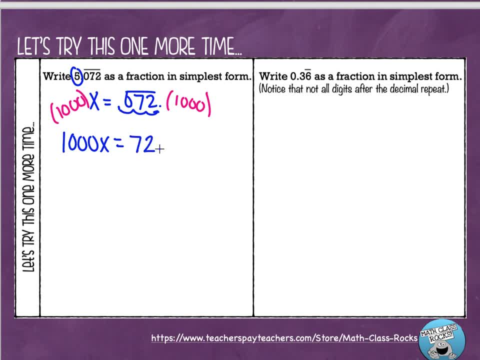 it's going to put it at the end. So I'm going to end up with 72 point, And if I were to keep going and put some more numbers after this, I'm going to put it at the end. So I'm going to put it at the. 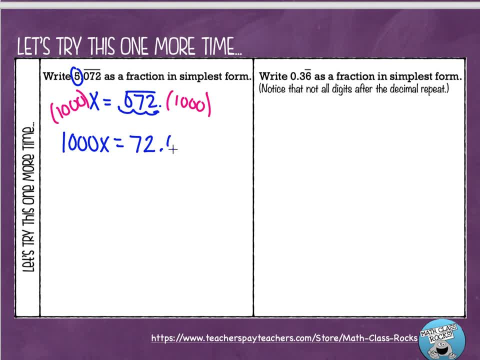 end of this decimal point. Since this is repeating, it would just be a 0.072 again, right? Because this is 0.072, 0.072, 0.072.. All right, the next step is I'm going to subtract out this original equation, So I'm going to write: 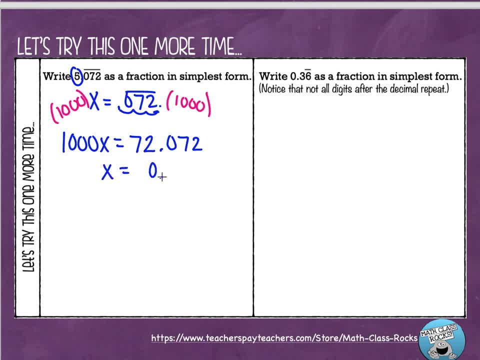 it underneath. I'm going to line up my decimals here And I'm subtracting this whole thing. That's going to give me 999x equals. this part here, right is going to cancel out, So I'm just left with 72.. And that's exactly what. 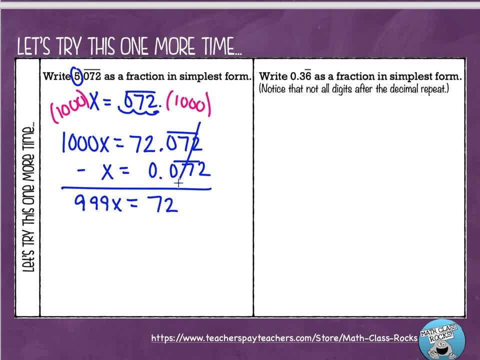 we wanted, right, We want that repeating decimal to go away. I'm going to divide each side by 999. And that's going to leave me with: x equals 72 over 999.. Now, again, I want to simplify this. 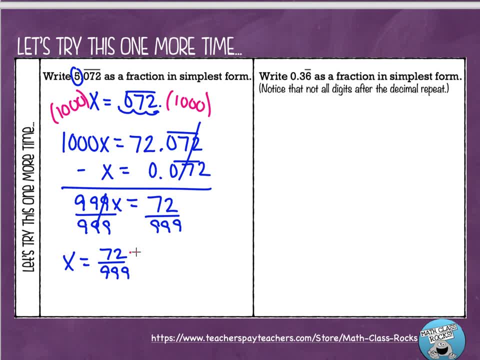 right. So I say to myself what would go in evenly to both of these, And again it's going to be 9.. 72 divided by 9 equals 8.. And 999 divided by 9 equals 111.. So 8 over 111.. However, let's not forget about this 5 up here. 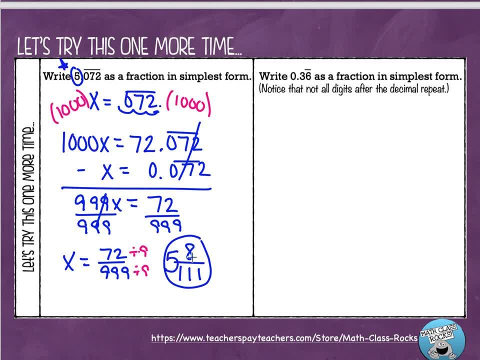 right, So I have to bring that 5 down And it's 5 and 8 over 111.. Right, And we just saved that 5 for the end, because there's really no point in doing the whole equation with that 5 in it. That's a whole number, So we can just do the decimal part. 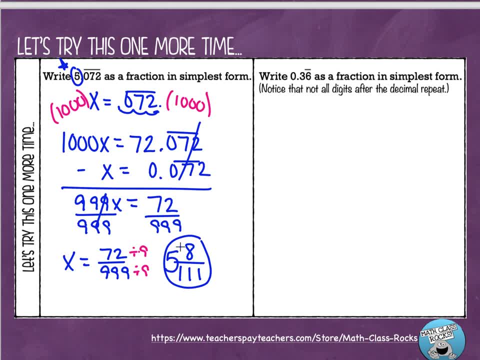 figure out what the decimal would be as a fraction and then just put the whole number in front at the end. It just was a little shortcut to make our life a little easier. Okay, this last one. now. This one is a little bit stranger, right? So I'm going to start out. 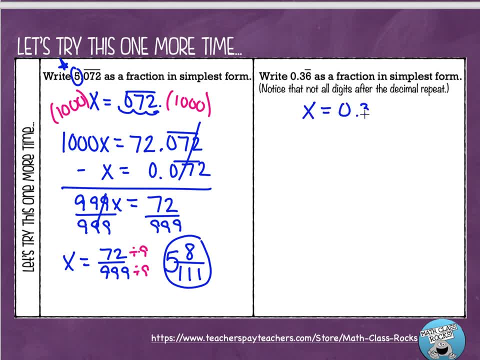 by writing my equation: x equals 0.36, and the 6 is repeating. Okay, we're going to multiply each side by 10, right, And remember, the exponent on the 10 is the number of digits that repeat. Well, only one number is repeating, right, This 3 isn't. 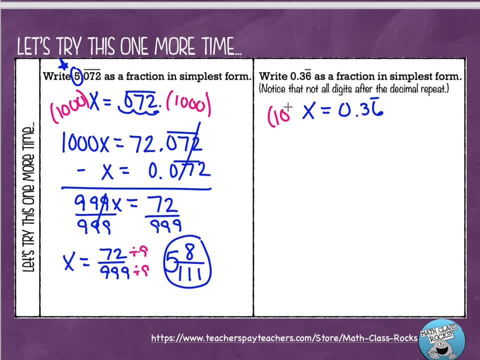 repeating just the 6.. So that means I'm going to multiply each side by 10.. Right, Don't mistakenly multiply each side by 100.. Only one number is repeating. Okay, so this is going to be a 10x on the left side. 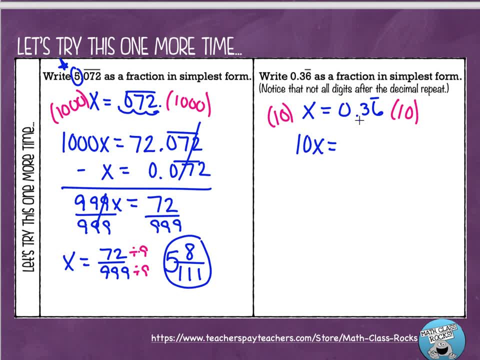 equals, And I'm going to multiply this side by 10.. 10.. So I'm just moving the decimal point over one time. So this is going to be 3.6, right, And that's a six repeating. So if I wanted to add any more digits here, I would just keep adding sixes. 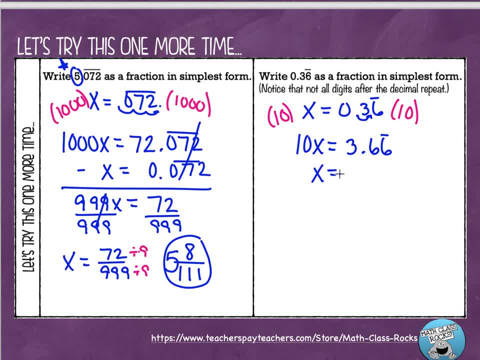 Okay, now we're going to subtract out this original equation: 10x minus x is 9x, And when I subtract this, I'm going to get 3.. I'm going to get 0.6 minus 3 is 3.. And these two repeating sixes cancel out right. See how that works. We always want that.